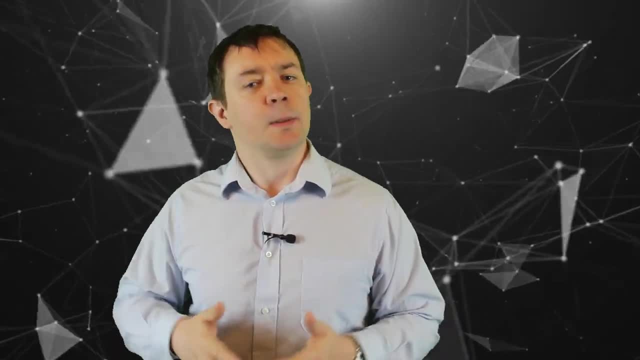 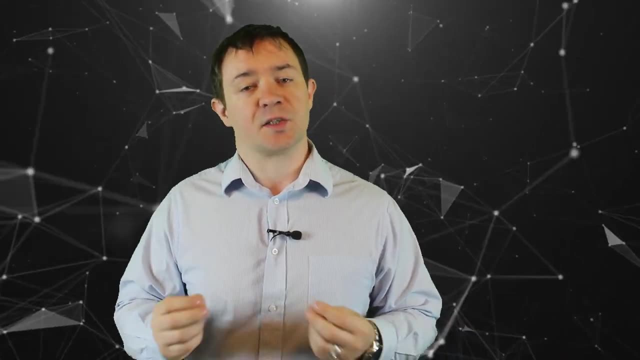 These rewards tell the agent what's good and bad, and the agent uses some algorithm to try to maximize rewards over time. In practice, what we get is a sequence of decisions by the agent, and each decision doesn't just influence its immediate reward. 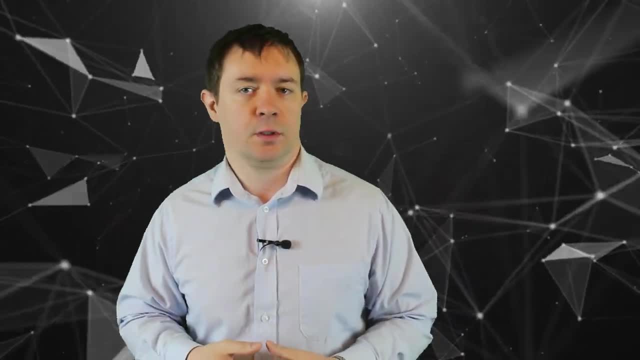 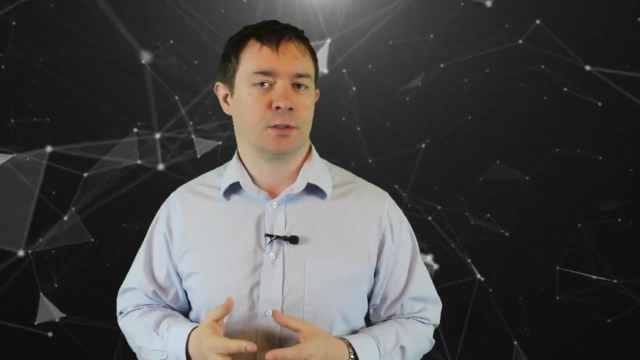 rather, each decision influences the outcome, All future rewards. In mathematical terms, we have a sequence of states, actions and rewards that one could call a decision process, If each state in this process is purely a function of the previous state and action of the agent. 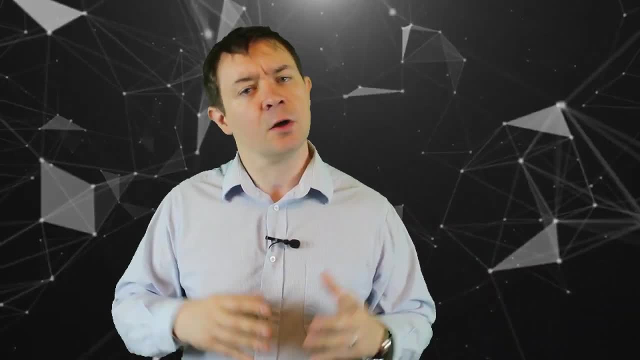 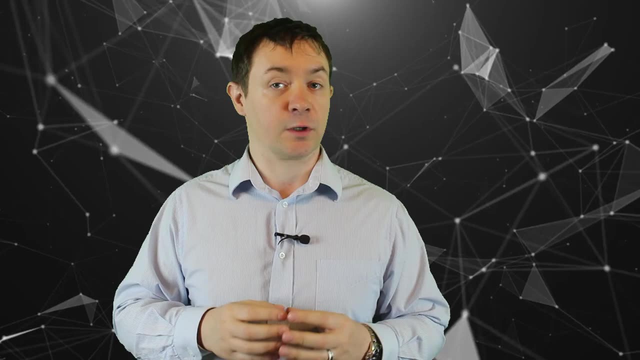 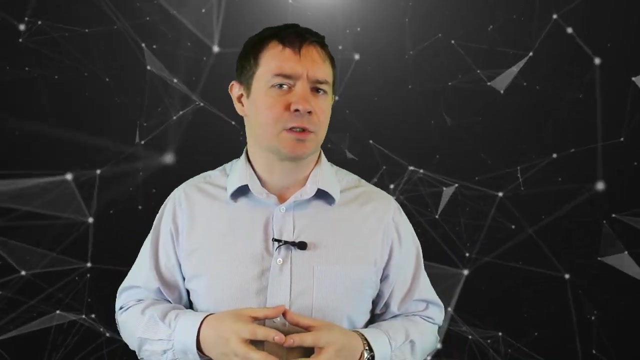 then this process is called a Markov decision process, or MDP for short. These are an idealized mathematical abstraction that we use to construct the theory of reinforcement learning. For many problems, this assumption can be broken to various degrees. How much that really matters is often a complicated question. 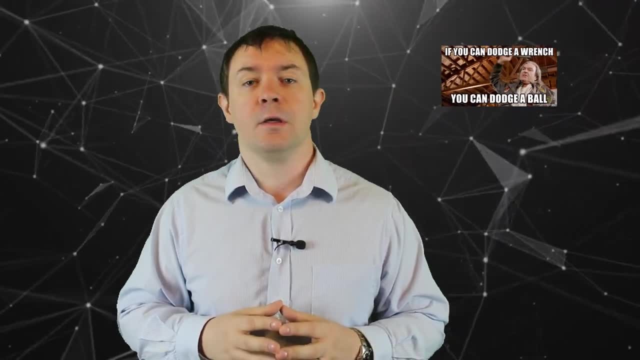 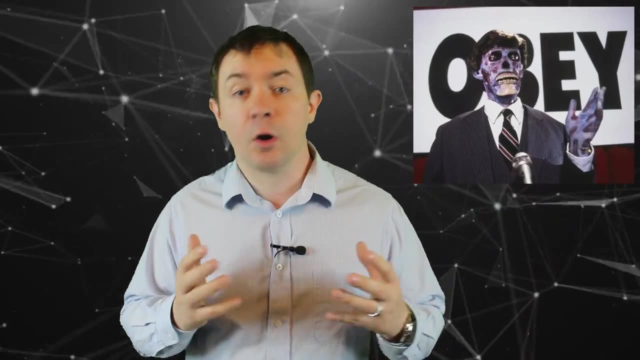 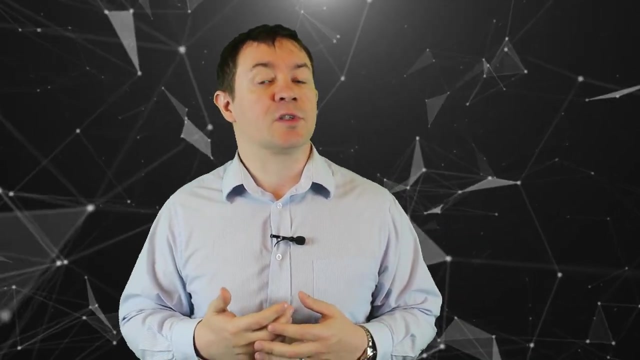 and one we're just going to dodge for now. Regardless, in most cases, the assumption that a process obeys the Markov property is good enough, and we can use all the resulting mathematics for reinforcement learning problems. By now I've said that a reinforcement learning agent seeks to maximize rewards over time. 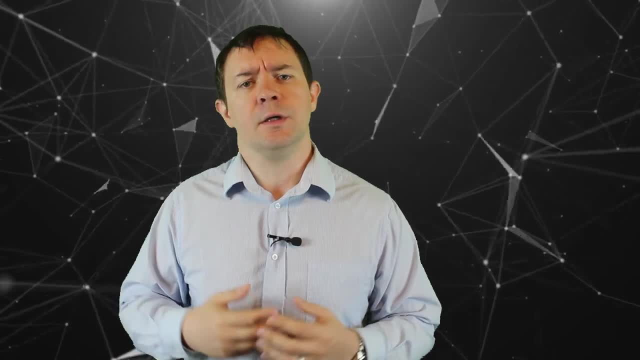 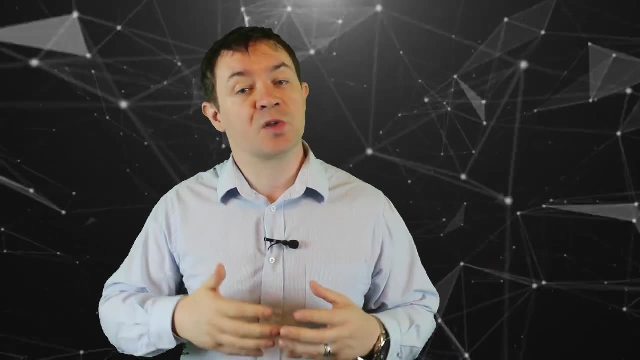 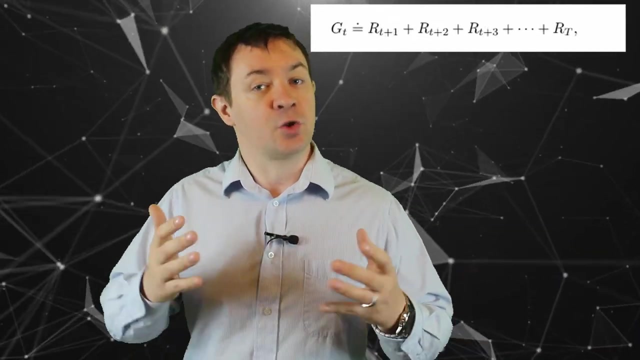 so how does this fit into a Markov decision process? From the agent's perspective? it receives some sequence of rewards over time and that sequence of rewards can be used to construct the expected return for the agent, Then the return at some time. step t is just the sum of 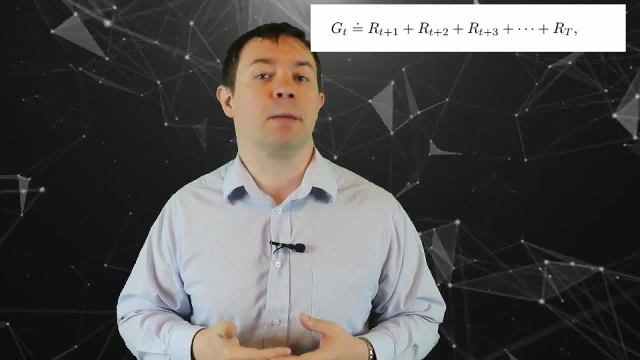 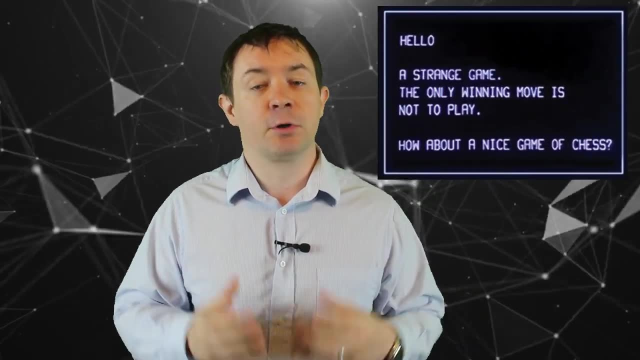 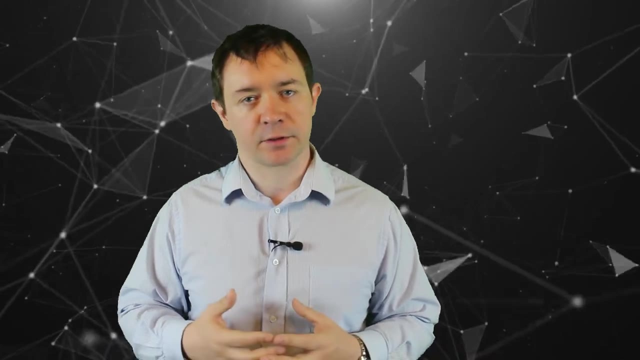 the rewards that follow all the way up to some final time, capital T. This final time step naturally introduces the concept of episodes, which are discrete periods of gameplay that are characterized by state transitions, actions and rewards Upon taking this final time step. 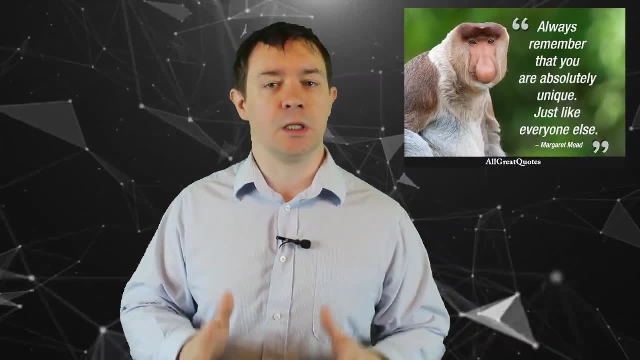 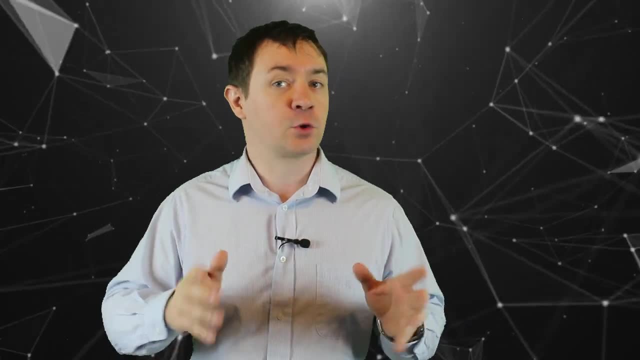 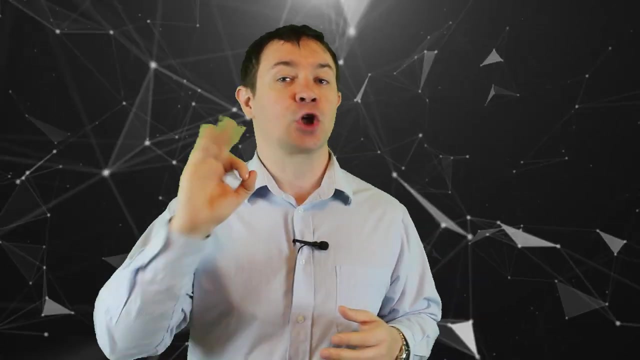 the agent enters some terminal state which is unique. This means that no matter how we end the episode, the terminal state is always the same. No future rewards follow after we reach the terminal state, so the agent's expected reward for that terminal state is precisely zero. 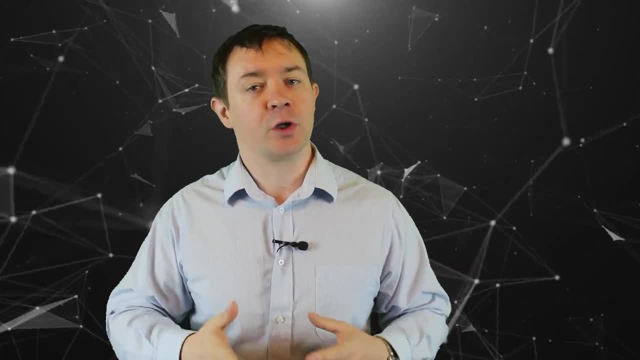 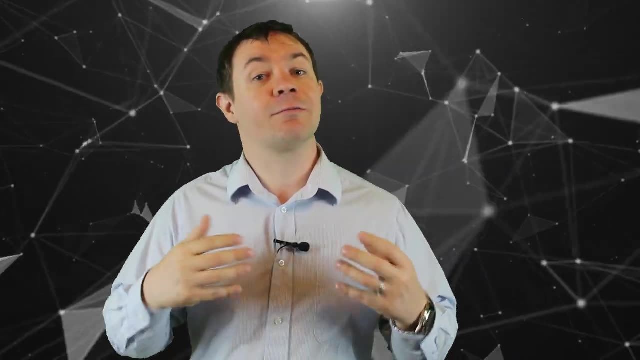 With a bit of creativity, we call tasks that can be broken into episodes episodic tasks. Of course, not all tasks are episodic. Many are, in fact continuous. This is a bit of a problem, since if the final time step is at infinity, the total reward could. 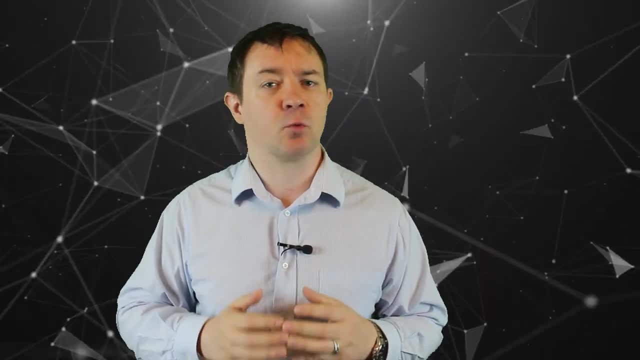 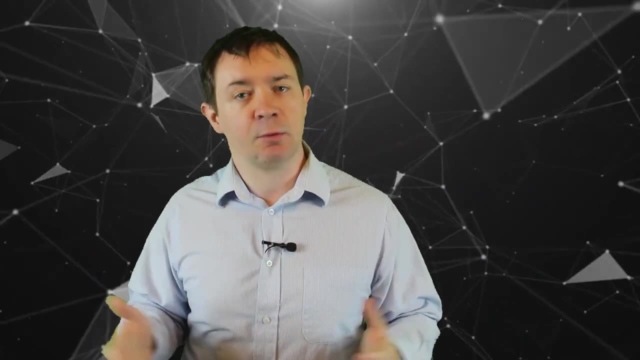 also be infinite. This makes the concept of maximizing rewards meaningless, so we have to introduce an additional concept. The fix- and we use this for both episodic and continuing tasks- is the idea of discounting. This basically means the agent values future rewards less and less. 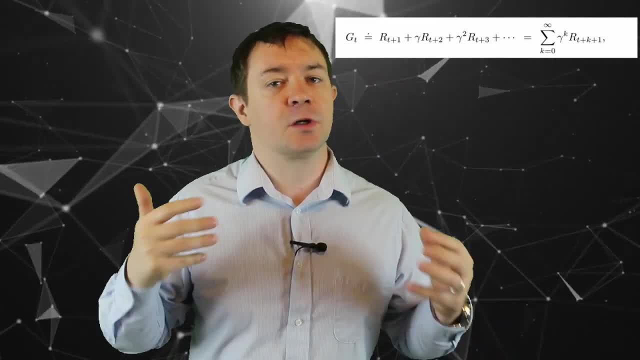 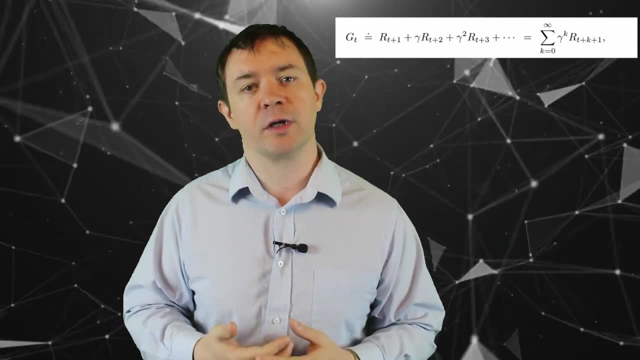 This discounting follows a power law where each time step results in more and more discounting. This hyperparameter gamma is called the discount rate, and you've no doubt seen this before in our videos on reinforcement learning. If you use this form for the expected, 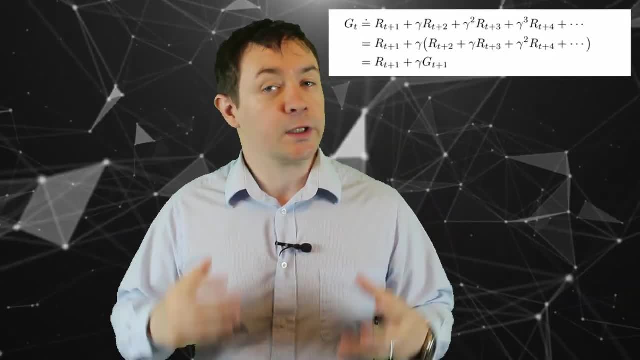 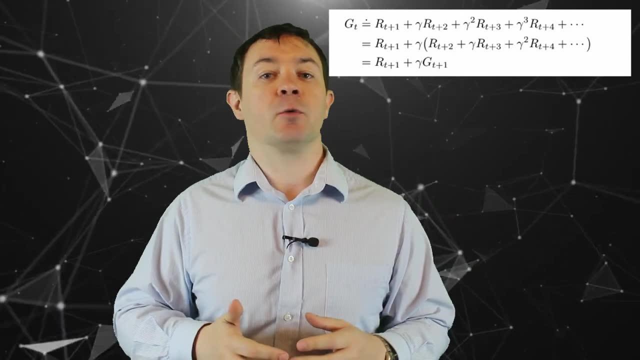 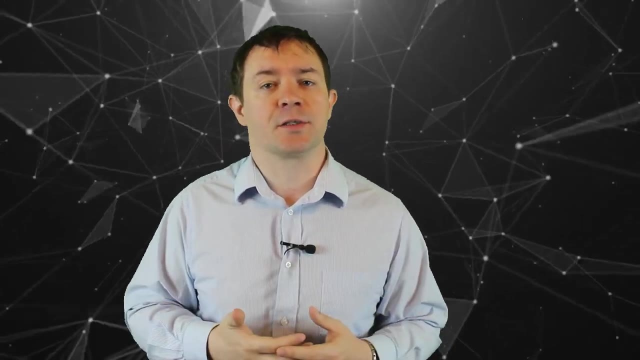 return and do some simple factoring, you derive a really useful fact. There is a recursive relationship between rewards at subsequent time steps. This is something we'll exploit constantly in reinforcement learning. So we have an agent that is engaged in some discrete processes. 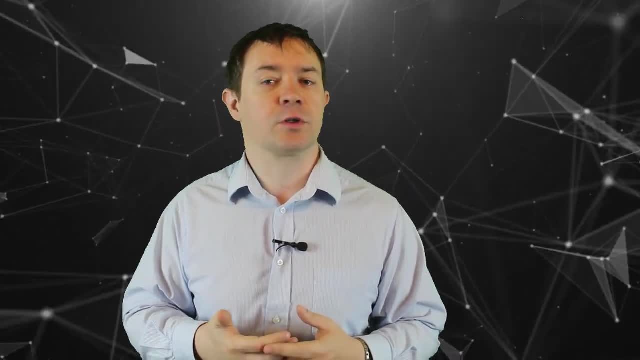 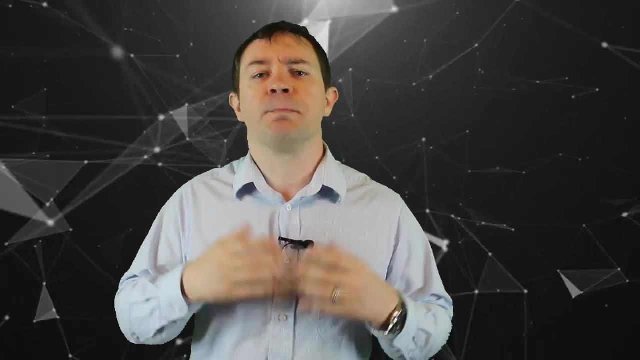 receiving rewards and trying to maximize its impact. This is an agent that is engaged in some to maximize its expected future returns. If you remember from the first lecture, the algorithm that determines how the agent is going to act is called its policy, Since the agent has a set of defined rules for how it's going to act. 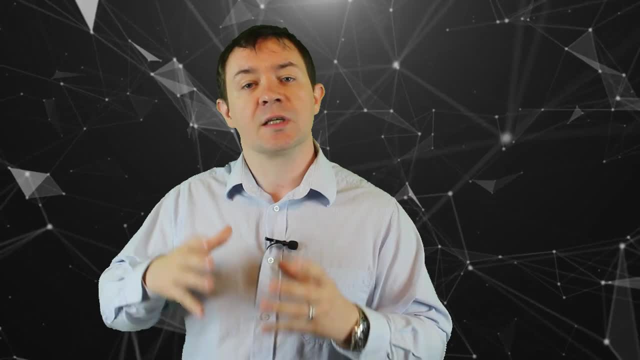 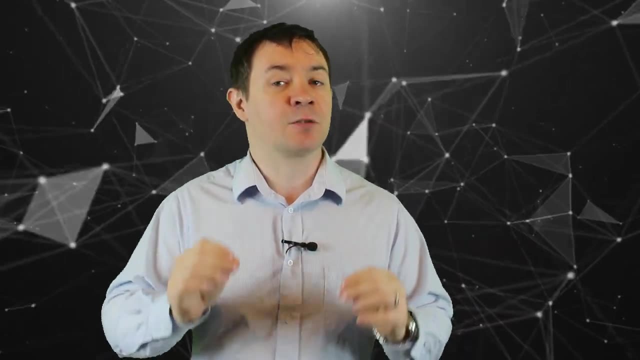 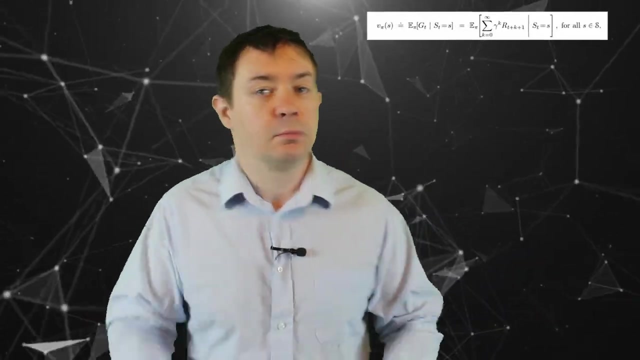 in any given state. it can use a sequence of states, actions and rewards to figure out the value of any given state. The value of a state is the expected return when starting in that state and following the policy. It's given formally by the following equation: In some problems like, say, Q-learning, we're 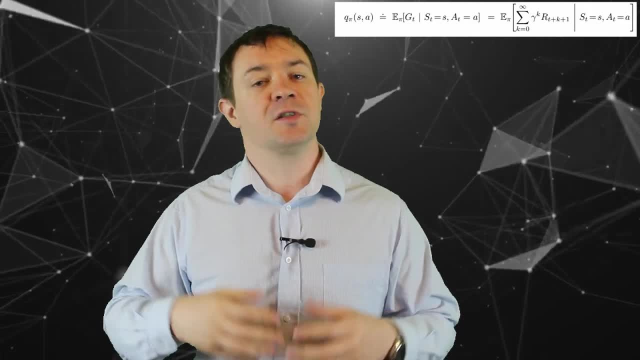 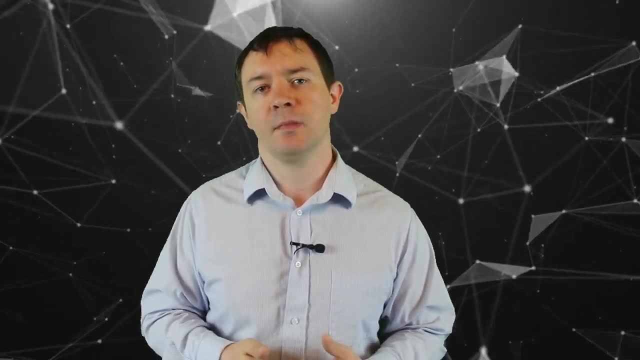 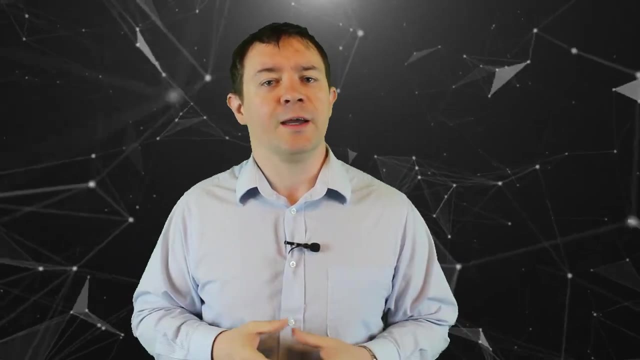 more concerned with maximizing the action value function, which tells the agent the value of taking some action while in some given state and following the policy thereafter. Remember how I said we can exploit the recursive relationship between subsequent returns. Well, if you plug that into the 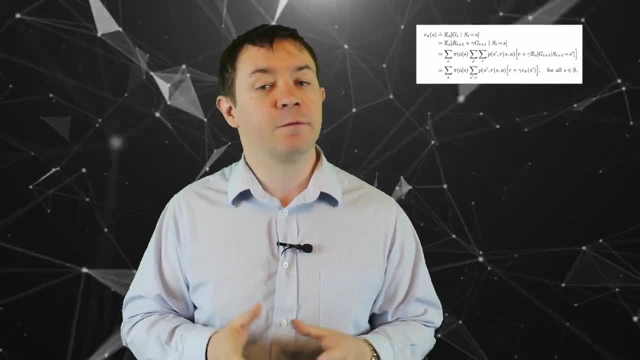 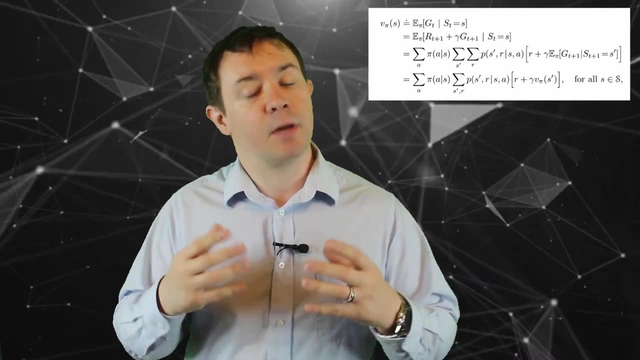 expression for the value function, we actually discover that the value function itself is defined by the action value function. This is called the Bellman equation from the first module, and it's the quantity many algorithms seek to maximize. The bellman equation is really an expectation.